this. if it's true, i would be certain to land on yellow, entonces esta light green, orange, gray and actually orange. Here we go in correct order. we can ourselves clean up each color. i need to just have one in order to determine what color to land on The quizzes지. 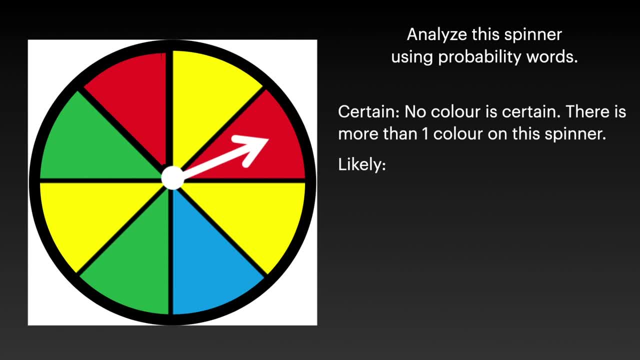 this question by seeing which color is on the spinner most. As you can see, there are three yellow spaces on this spinner. Yellow appears the most on the spinner, so it is most likely that the spinner will land on the yellow space. Equally likely Now, which two colors are equally likely to be landed on if I were to spin. 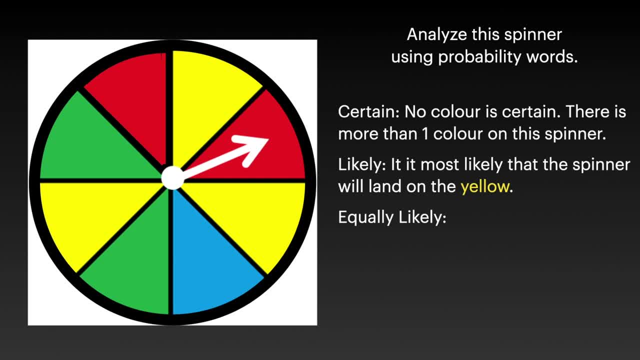 this spinner. We need to find two colors that show up on the spinner- the same amount. Looking at the green on the spinner, there are two green spaces. and looking at the red on this spinner, there are two red spaces, So it is equally likely to land on. 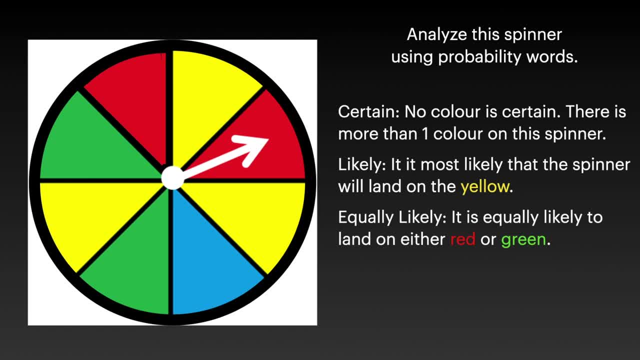 on the green space. red or green- Unlikely If I were to spin this spinner, which color am I unlikely to land on? Which color is on the spinner the least? Yes, blue. There is only one blue space on this spinner, which is less than all the other colors. So it is. 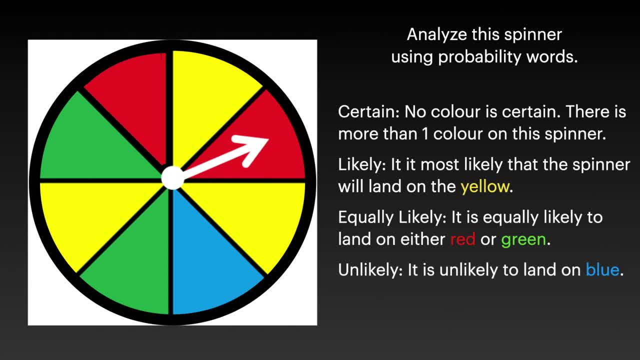 unlikely to land on blue. Finally, let's talk about the word impossible. If I were to spin this spinner, which color would it be impossible for me to land on? Now for this question, I could choose any color that I don't see pictured here. So 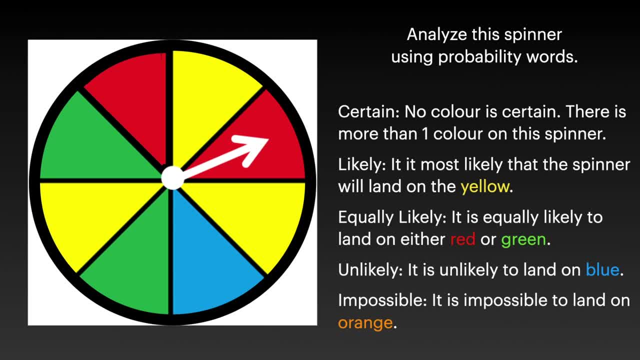 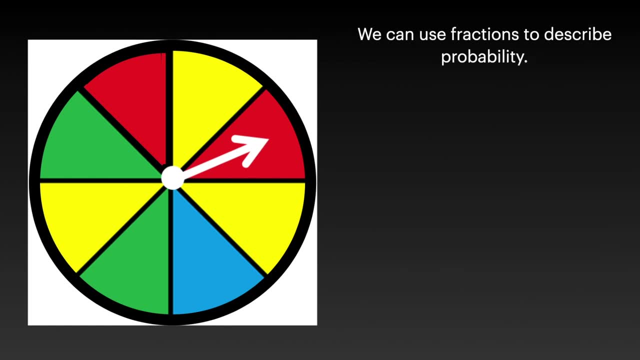 I've written that it is impossible to land on orange because there is no orange on the spinner. I could also say purple or brown or or black, whichever color is not pictured here. I also want to use this spinner to talk about how we can use fractions to describe probability. We just finished up our fractions unit, so I know. 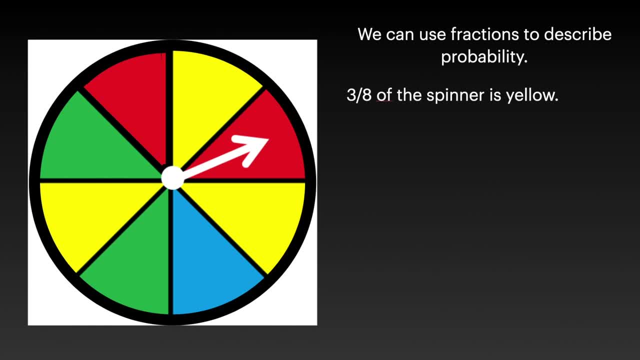 that you will all be experts here. Now, looking at the yellow on the spinner, I see that three spaces are yellow, So I can create a fraction. and I can say that three-eighths, because my spinner is divided into eight equal sections. three-eighths of the spinner is yellow, So I can write a.